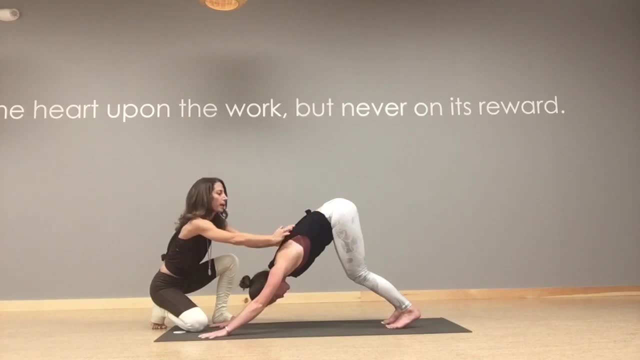 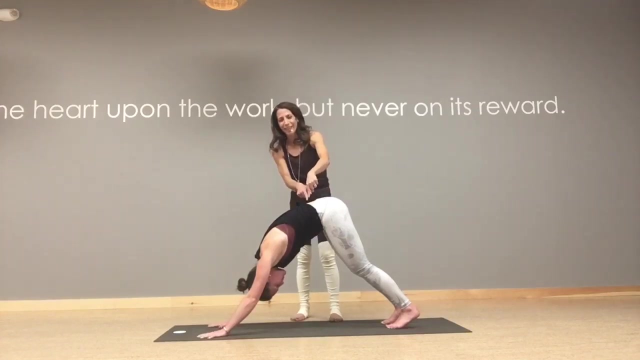 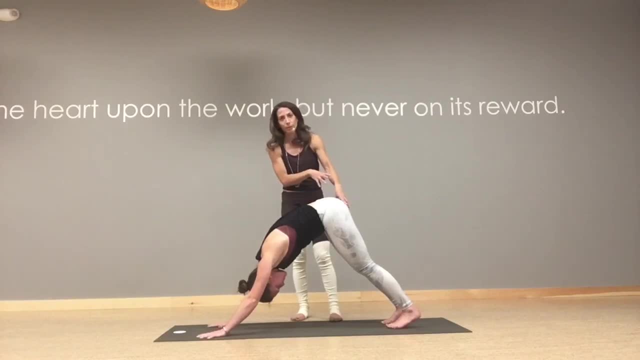 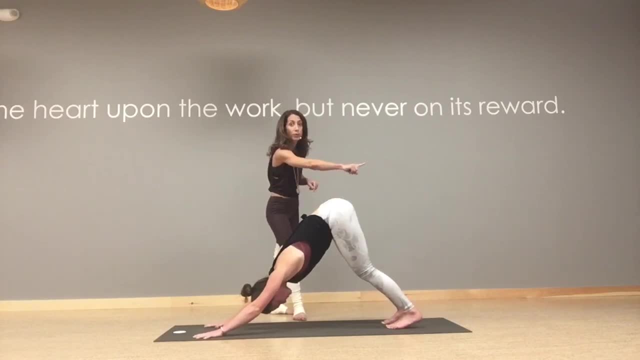 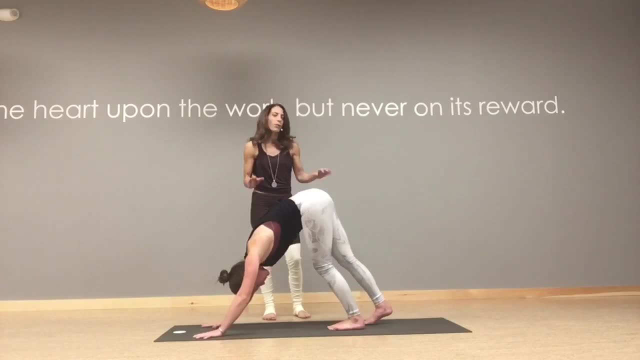 the posture, you want to lengthen the stance out a little bit. it's rare that I ever see anyone's heels down on the mat. I've been practicing over 20 years. my heels don't hit the mat, so you know. let go of this idea of getting the heels on the mat. take the nice, proper shape of the pose which 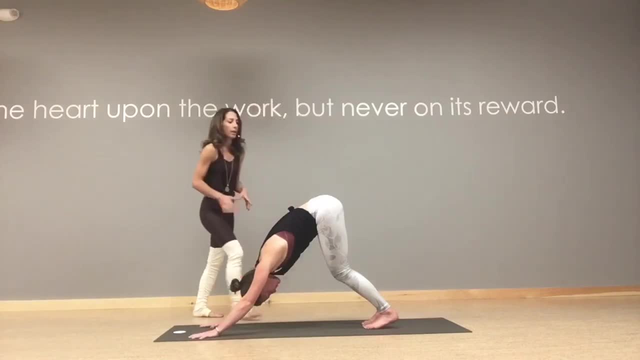 is a more V shape in the body. so that's our downward facing dog. just take one more. look: long spine, sit bones lift up and then the backs of the legs will start to release. from here we'll talk about plank pose. so we'll talk about transitioning afterwards. right now I'll just 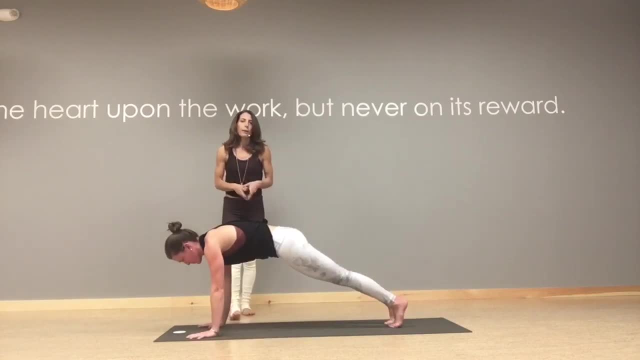 have Katie come into plank pose. so your markers for plank pose is that the feet, they can be together, but we're going to practice it hips distance apart to create a lot of strength in the body. so feet, hips distance apart, and the heels stack right over the toe mounds and it's 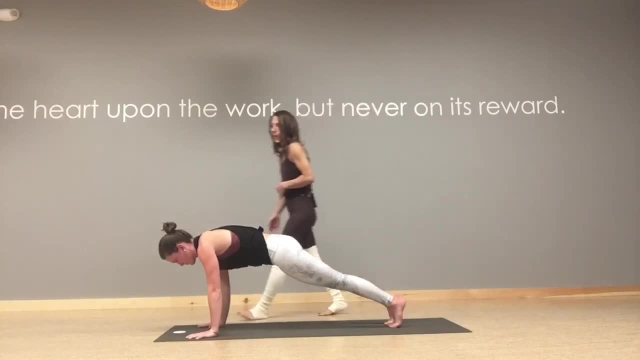 okay to shift your feet around to get that alignment. the other marker we want to look at is that the shoulders stack right over the wrist so Katie can actually move her shoulders back and forth, and then we'll talk about plank pose. so we'll talk about plank pose. 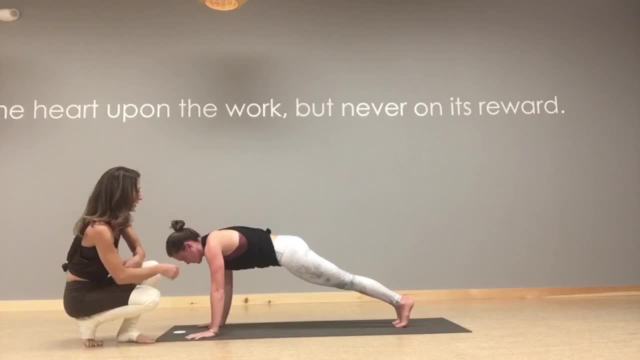 just a little bit and notice she's shifting her feet to accommodate that shift. hands are still the same, triceps hugging in shoulders still wrap back and around. but there's this also, this element of pushing the floor away and spreading a little bit the shoulder blades away. core nice and engaged. 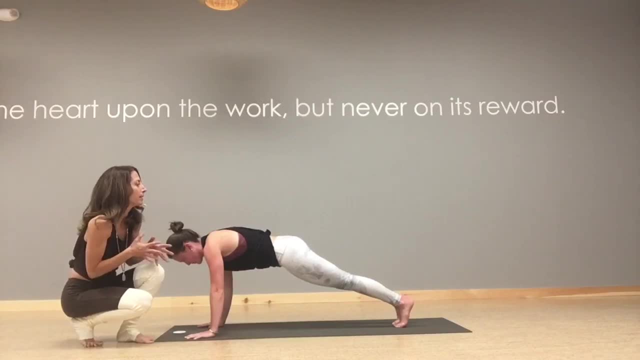 so this is a great pose to build course stability, because all of the muscles have to work here to keep the spine long in the pelvis stable. you also can use your legs a lot, so squeeze the quads and then you're going to be able to stretch your legs, and then you're going to be able to. 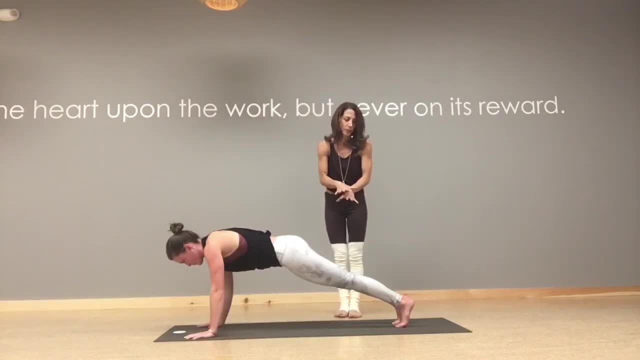 do a little bit more of a plank pose. so next up we have Chaturanga. this is a hard pose to hold, so I'm going to ask Katie to come down to our knees for a second so we can talk about the alignment and the arms. so, Chaturanga, the most important thing is that the arms are at a 90 degree angle. 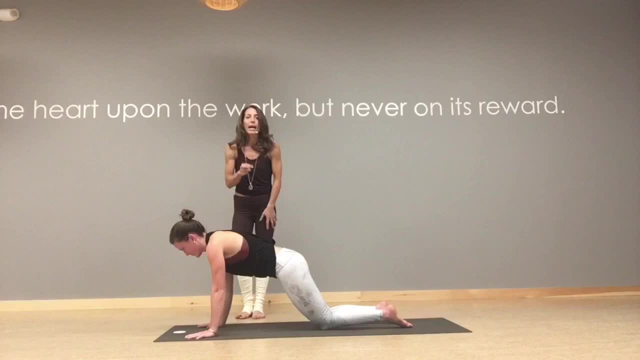 and many people cannot make that shape with their knees off of the ground and that's why we often cue to bring the knees down. it has a still going to work for the body. if you have a very serious пост and you have a little bit of a push back to the ceiling, that's not going to work for the legs. 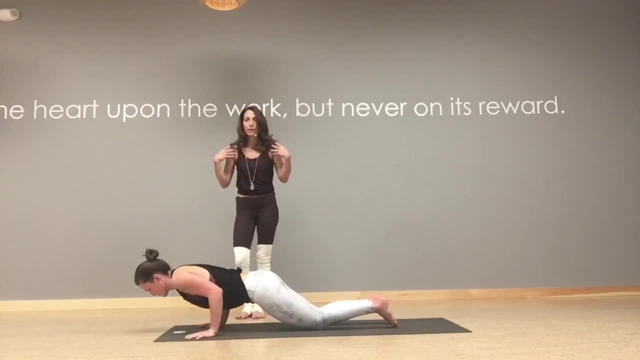 or the back and forth. now we're going to talk about the third part, the supra. so let's start with the, the right muscle group, which is your pecs and your deltoids and your biceps. so don't worry about the knees being on the ground. so shoulders line up to elbows- elbows. elbows stack over wrists- shoulder. 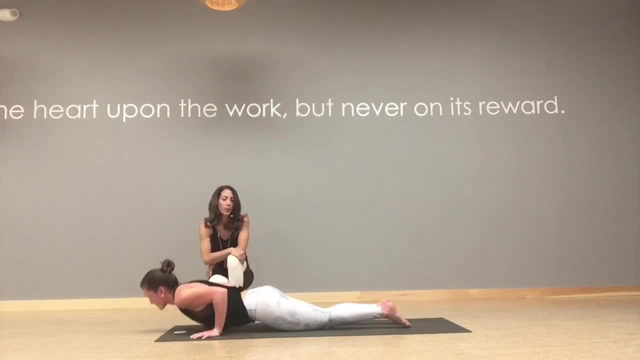 blades come towards the spine and you can go ahead and come on up or down. good, so chaturanga is another core strengthening exercise and also build strength in the arms. the legs are straight, I'll have you heard. take the full shape of the pose with the knees off the ground for a moment again. 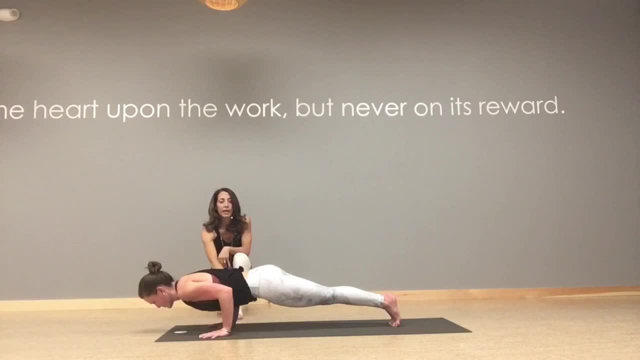 hands are the same. good, so nice 90-degree angle in the arms. long spine heels still stack over toe mounds. great, you can come on down. good. so next up we have coat. so Cobra pose and up dog. I want to take this moment to differentiate between the two, so we'll start with Cobra pose. 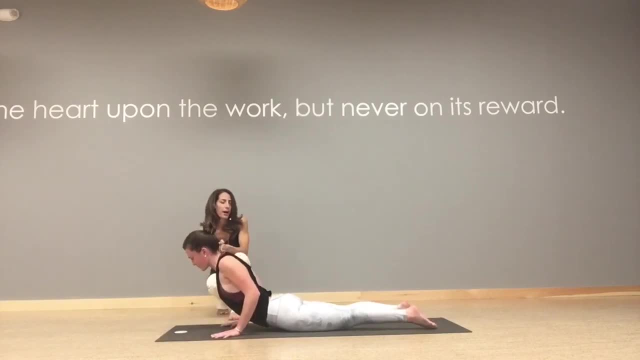 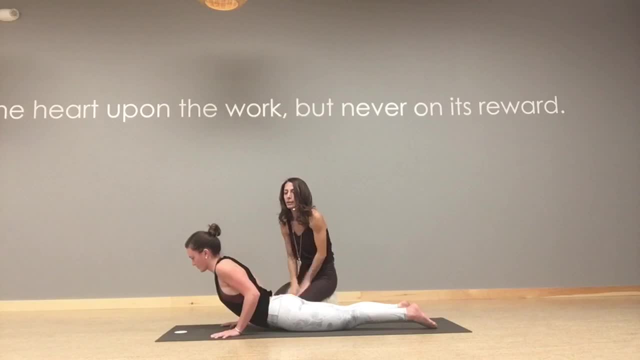 bent and the elbows are pointing towards the back of the mat rather than out to the side. if you can show out to the side, Katie, I see a lot of that. that internally rotates the shoulders, which is the opposite of what we want to do. so draw those elbows to point back. that'll automatically roll. 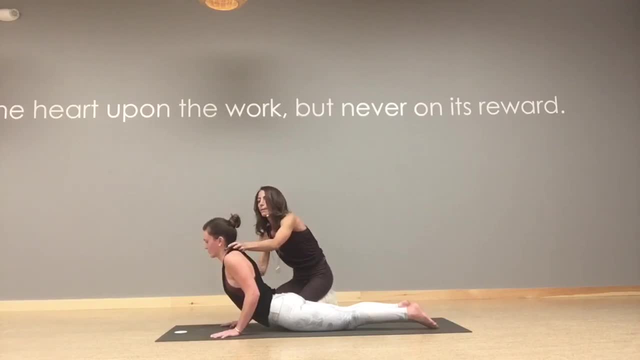 the shoulders forward and back, sternum shoots forward and then the base of the skull presses straight back rather than. can you look up like that's just overextending the spine. that's not very good for your cervical spine. so the gaze is more forward. press the soft palate. 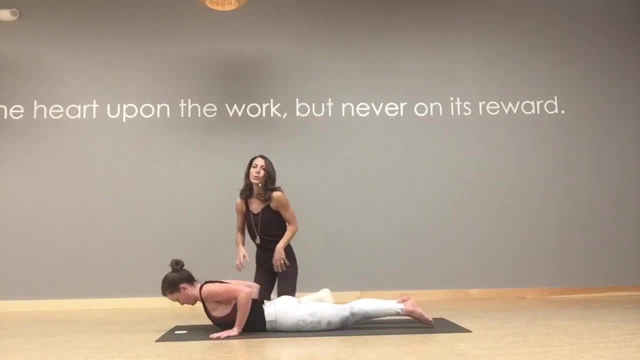 straight back. good, so that's your Cobra pose. shoulder blades come towards the spine for up dog. this requires a little bit more back flexibility and strengthen the arms. all everything's off the mat except the tops of the feet and the hands and the arms. straighten the shoulder blades come. 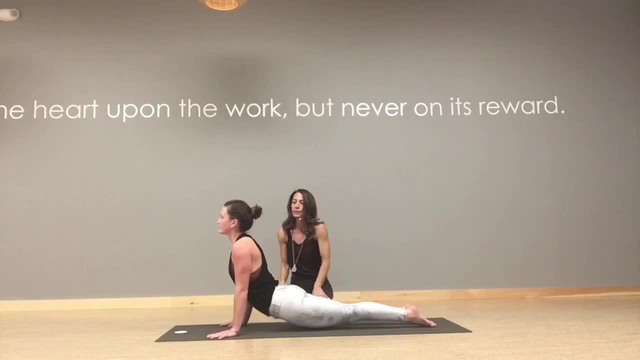 towards each other. you can see it's a pretty deep back bend. so you want to be nice and open for your up dog good, and then come on down, Katie. that's a lot of information. we're going to talk about linking all of those together so you can think of your flow as one continuous nice movement in this. 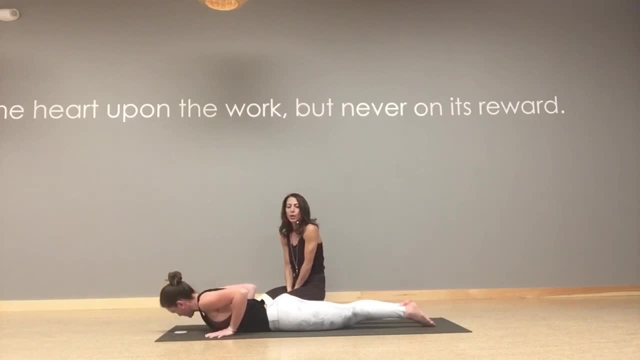 beautiful sequence that creates strength and flexibility. so, starting in downward-facing dog, good, nice v-shape in the body: feet, hips, distance apart. she'll inhale and wave forward from the very base of her belly. good, and notice she's shifting her feet and finding that alignment in her body. 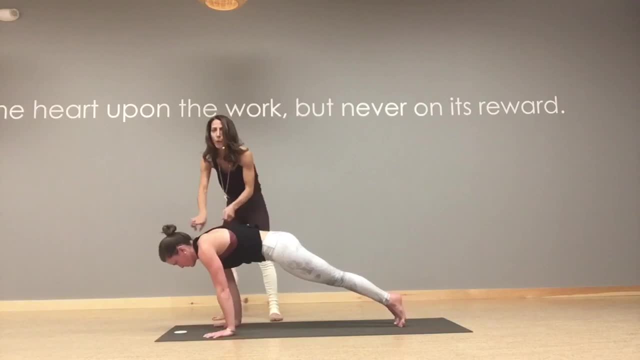 now super important. you have to shift way more than you're supposed to and you're going to want to stay in that 90-degree angle of the arms when you bend. good, now notice the shoulders. never dip down as she transitions to up dog and then curl the toes. you can go one or two at a time, we'll